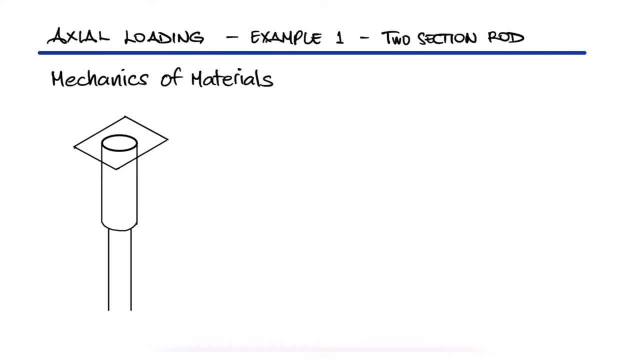 Two brass rods, AB and BC, will be braced together at B and subjected to the loads shown while suspended from a support at A. If the diameter of rod AB is 50 millimeters and the diameter of rod BC is 30 millimeters, what is the average normal stress at the midsection of rod AB and 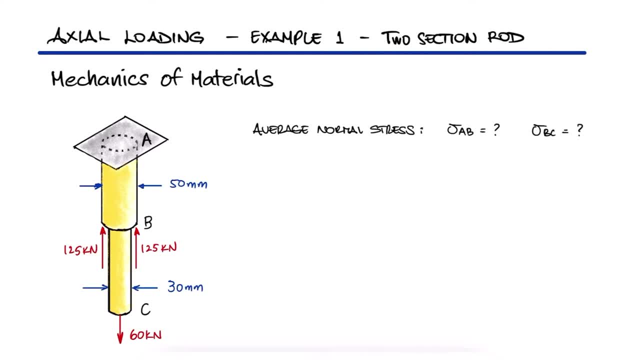 rod BC. This is the first example for the axial loading main video link below. To calculate these normal stresses we'll use the expression that we used in that main video. To find the forces FAB and FBC, we'll perform a cut somewhere around the midsection of both rods. 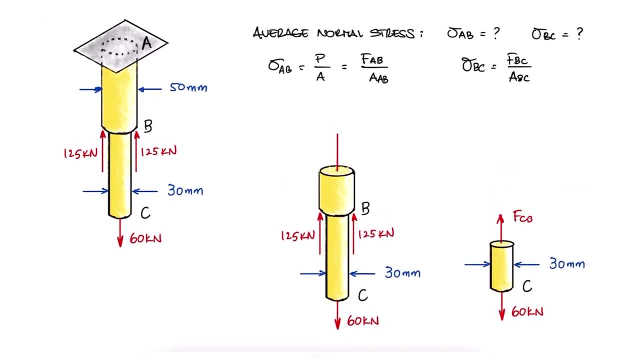 Completing the free body diagrams with the internal force at the cuts will allow us to write a sum of forces and solve for the force variables we need. And notice that the direction of the rod BC will be the same as the force at the midsection of both rods And notice that the 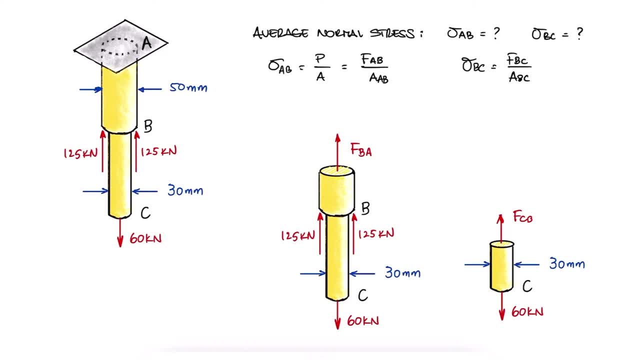 direction of the vectors I used are such that if the value for the forces is positive, the stress will be positive and therefore tensile, and if the value for the forces is negative, it means that the vector should have been pointing in the opposite direction, making the stress a compressive stress. 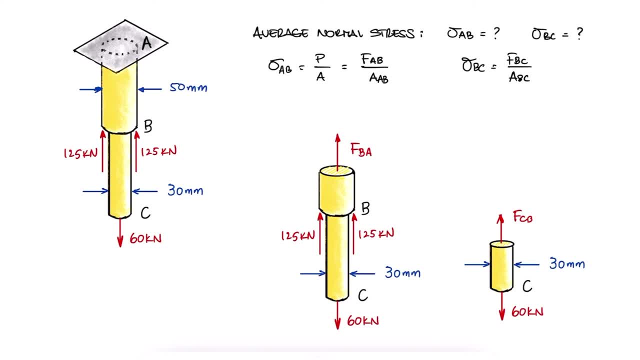 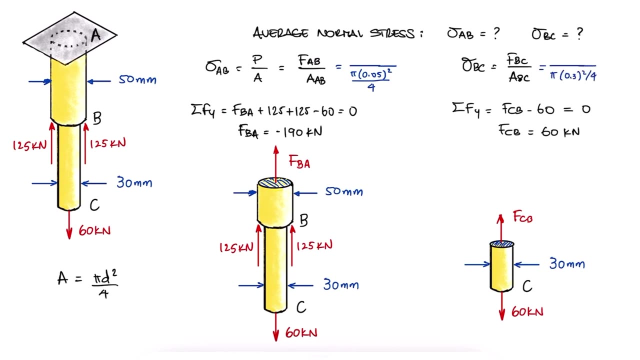 which is consistent with the negative numerical value. The sum of forces reveals that FCB is equal to positive 60 kilonewtons and that FBA is equal to minus 190 kilonewtons. The cross-section areas are those of a circle and the force values should be substituted in newtons. 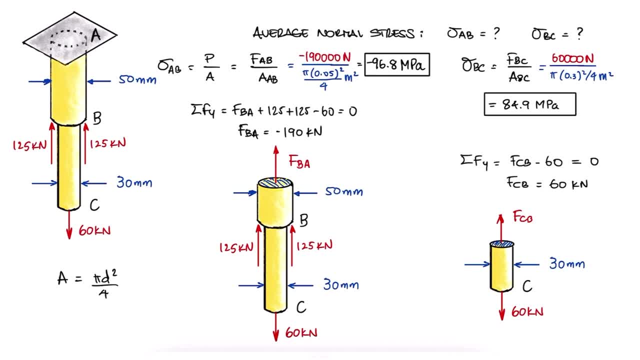 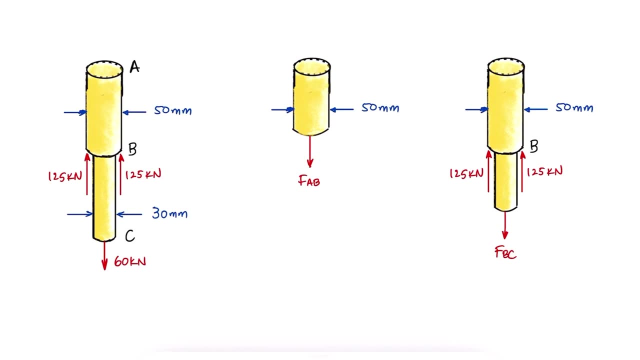 to have consistent units. Notice that rod AB is under compression and rod BC is subjected to tension. Additionally, notice that the cut can be performed from the bottom, like we just did, or from the top, and we would obtain the same values. 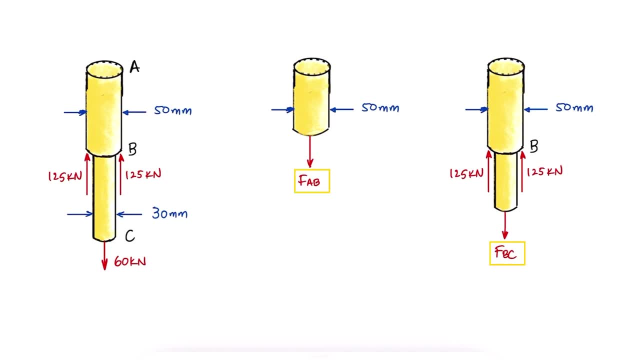 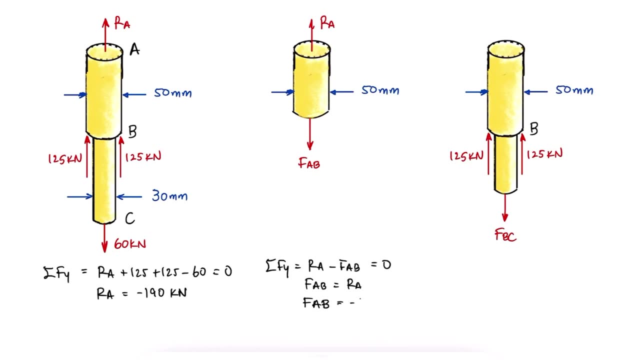 However, to solve for FAB and FBC in this case, we would first need to find the reaction force at A. FAB will still be equal to minus 90 kilonewtons and FBC equal to 60 kilonewtons, But of course this requires that extra step and being extra careful about being